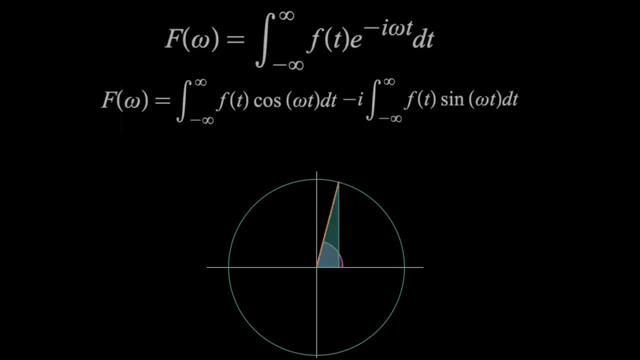 so we need to think of this more like the unit circle, where the phase can be positive or negative, or greater than 90 degrees, and so on. This will tell us if any of those areas are in fact negative, which we'll see later. 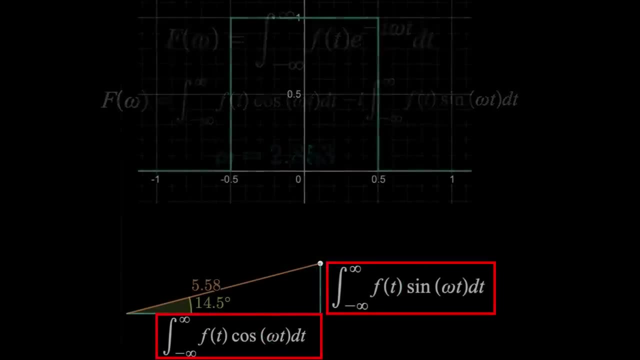 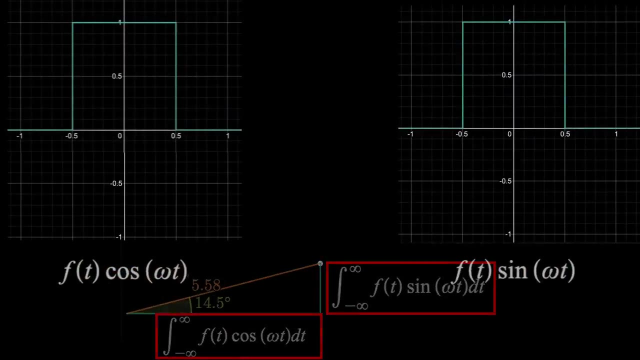 But here let's just go to an example. I'll put the rectangular function back on top here. but what we're going to do is multiply that by cosine of omega t and also sine of omega t. so we can see why this is the magnitude of the Fourier transform. 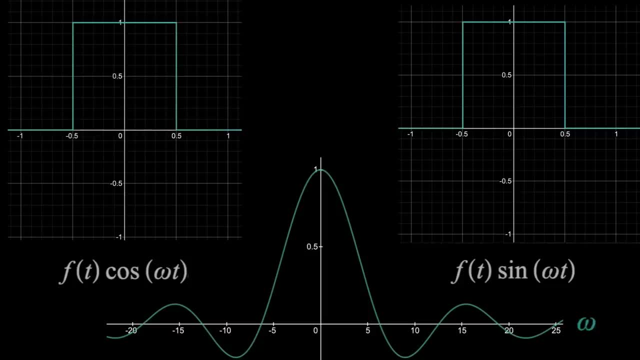 which is a function of omega. by the way, Making sure there's room on the screen was one of the tougher parts for this video, but I'll keep the rectangular function plotted on both the left and right, but use dots instead, while the trig functions will be solid. 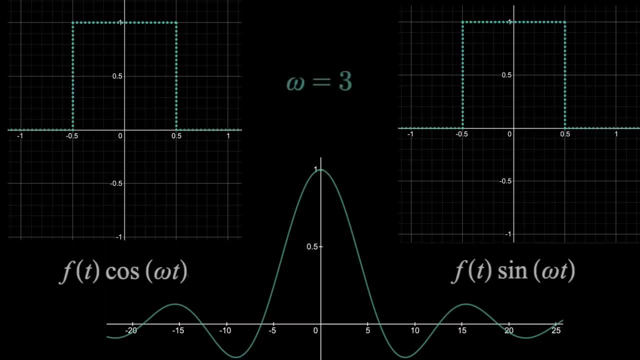 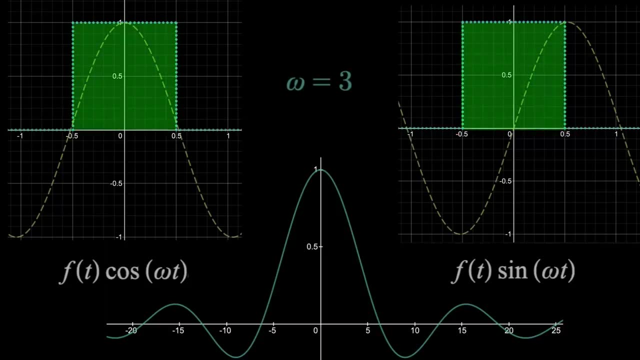 I'll start with. omega equals 3.. Cosine and sine of 3t look like this, But since our rectangular function is zero everywhere besides these regions, then multiplying the equations together leaves us with the same things just chopped off on the sides, as shown. 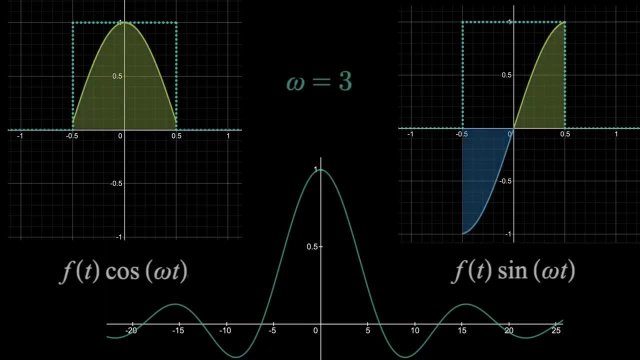 Now the Fourier transform says: find the area under these curves and just get the magnitude from there. Since areas beneath the x-axis are negative, then the plot on the right has an area of zero. The region on the left has an area of about 1.5.. 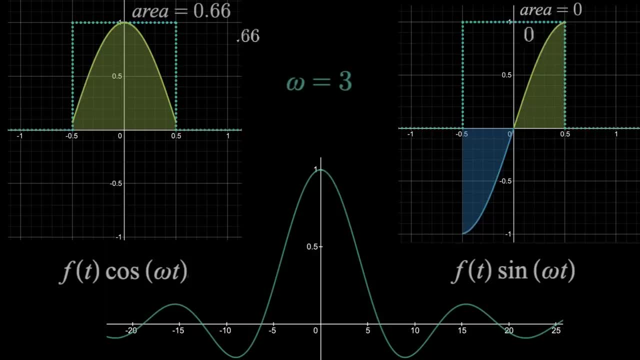 The area on the right has an area of about 0.66.. And the magnitude of these is, of course, 0.66.. No Pythagorean theorem needed when one side is zero, Which means at omega equals 3, the magnitude of the Fourier transform is 0.66. 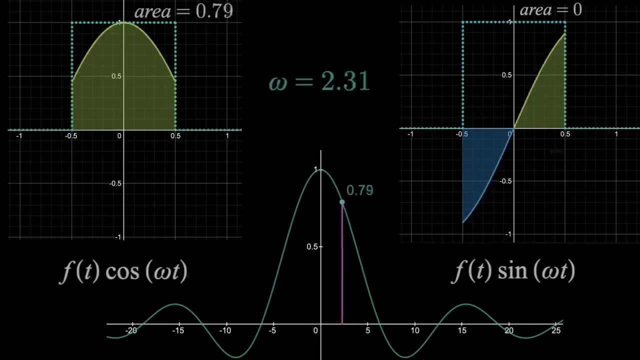 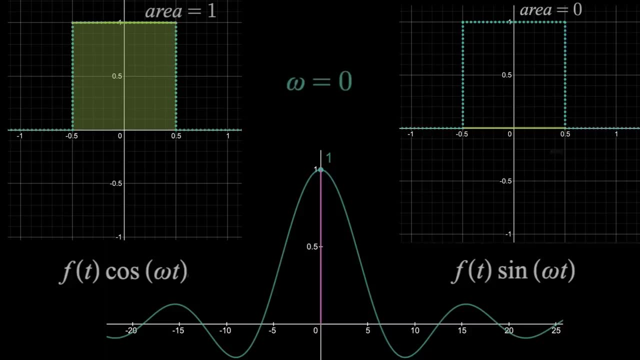 So all we need to do from here is sweep omega and keep track of those associated areas, and this will get us the entire Fourier transform magnitude. By the way, notice, as I rewind a bit, that the graph on the right always has an area of zero. 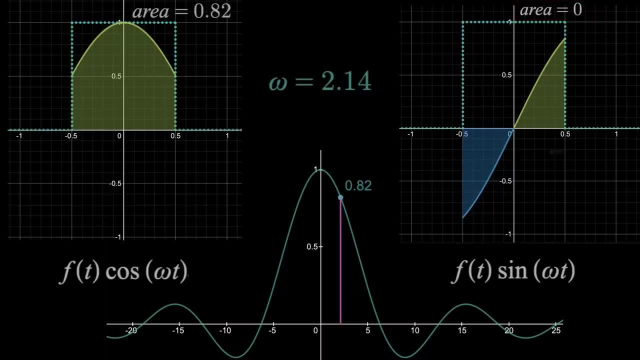 That will be the case for even functions symmetric about the y-axis, because the positive and negative areas will always cancel when multiplied by sine of anything t. So really we are plotting this area as a function of omega that entire time In this case. that's really all. the Fourier transform is 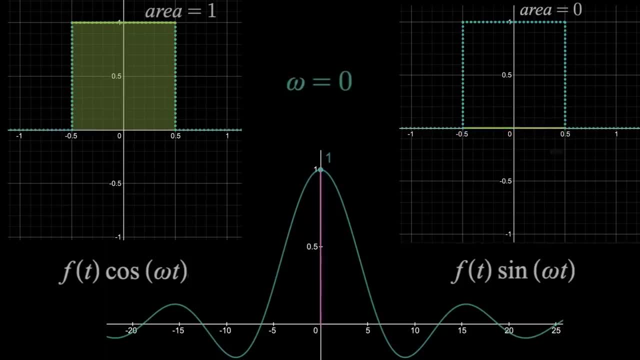 Let me also show you two points of interest. One is here at omega equals 0, because this y-coordinate actually tells us the area under the curve. The reason for this is when omega is 0, this here just puts the area below the curve. 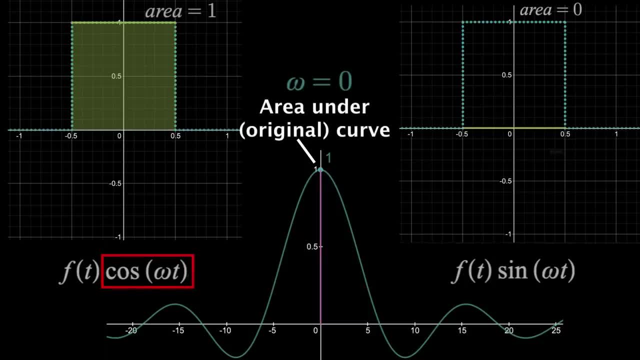 And the reason for this is when omega is 0, this here just puts: the area below the curve becomes one. so we have the graph of f of t and the function on the right becomes zero, regardless of what your f of t is. so we ignore that. this means we're just applying the area of f of t, the 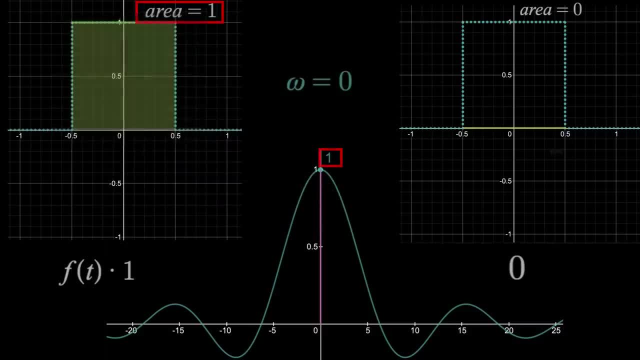 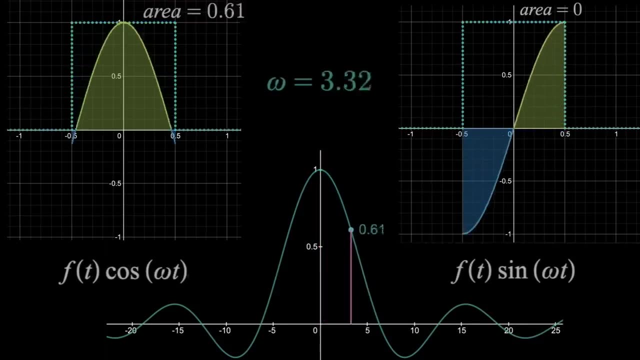 original curve. you can see that here with the original rectangular function and the area beneath it. then let's move to omega equals 2 pi, because that has a value of 0 on the magnitude plot, if you ever see a magnitude of 0. what that means is that if you multiply your original function by 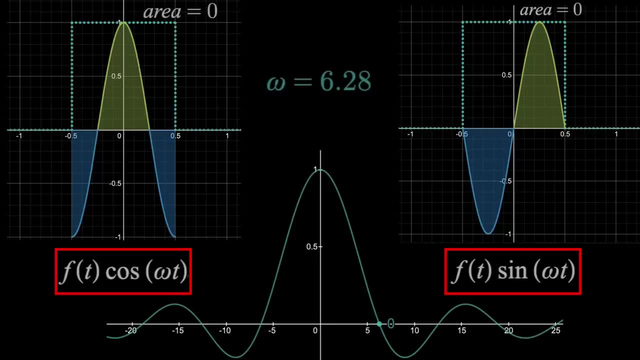 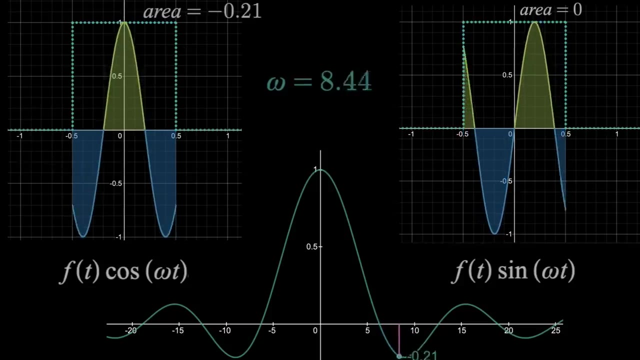 cosine or sine, with that angular frequency 2 pi. in this case, the area under both those curves will be 0.. this is where the left plot finally got enough negative area to cancel out the positive area. then, as we keep increasing omega, the area on the left oscillates from net negative to net. 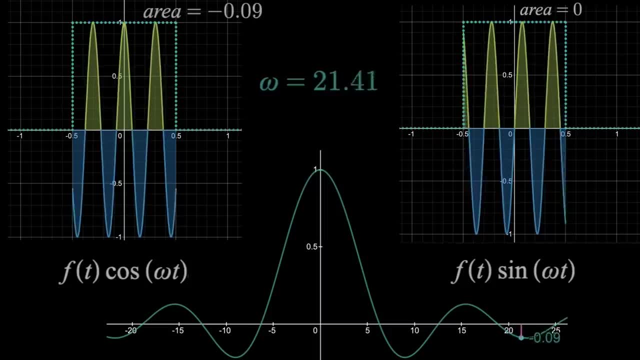 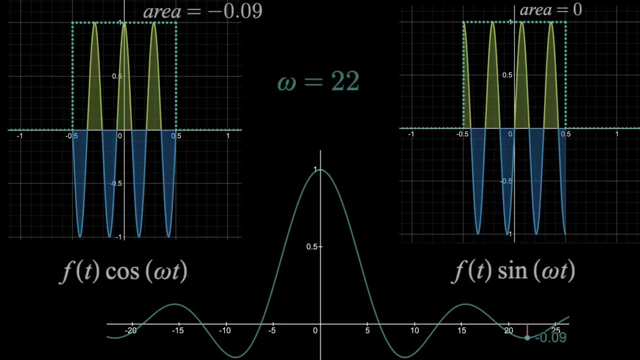 positive while converging to zero. so we've constructed the magnitude plot by just using real areas of real functions. didn't have to really think about a magnitude plot, but just using real areas of real functions. didn't have to really think about a imaginary numbers. to see the intuition here and just to summarize all that with a slightly more: 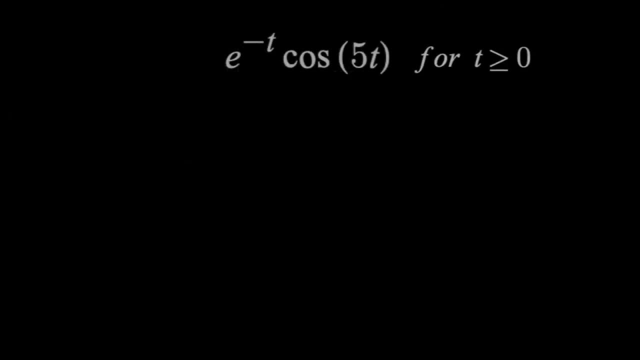 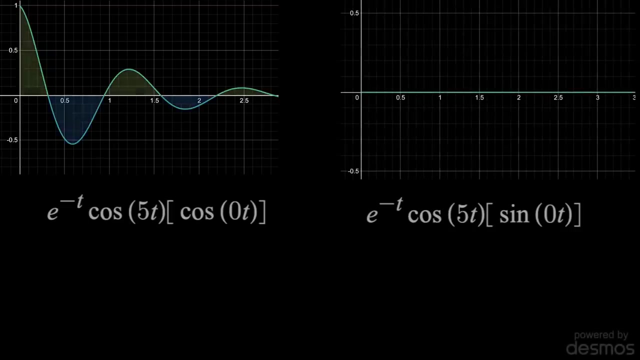 complicated equation. let's say this is our f of t. in order to find the fourier, transform, multiply that by cosine and sine of omega t, starting at omega equals zero, which leaves us with just the function itself, and y equals zero. then find the area under both those curves and. 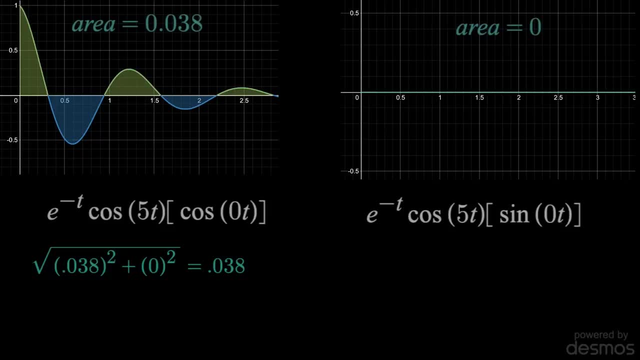 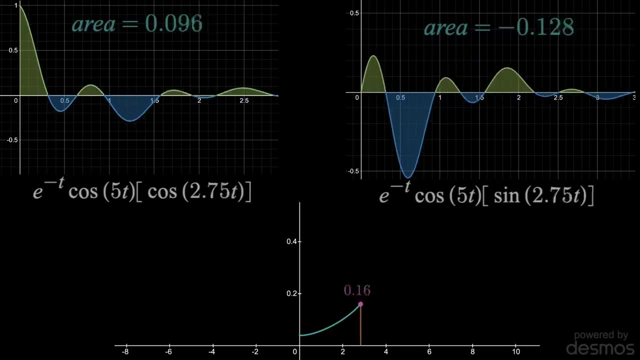 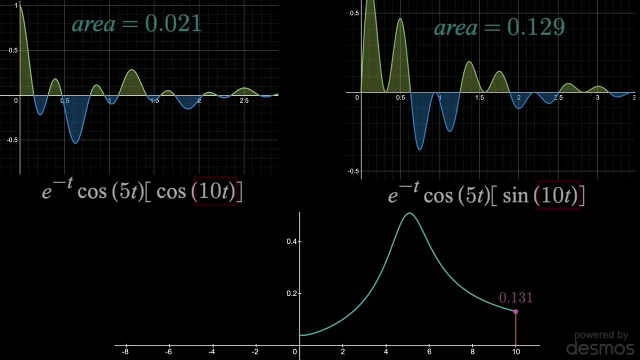 use the pythagorean theorem to get the magnitude and plot that point at. omega equals zero. then just sweep omega and keep track of that magnitude to create the fourier transform magnitude plot for any omega, like 10 in this case, you'll see that the magnitude of those areas is equal. 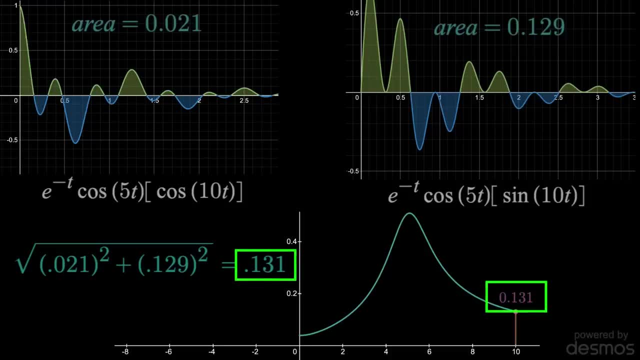 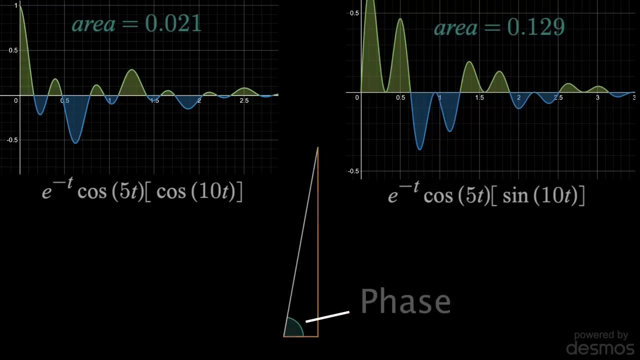 to the y coordinate on the bottom graph at that specific omega, and we see the same thing for negative values of omega. meaning this is the final fourier transform magnitude, and real quick. in regards to phase, remember that was just the angle in the triangle with side lengths equal. 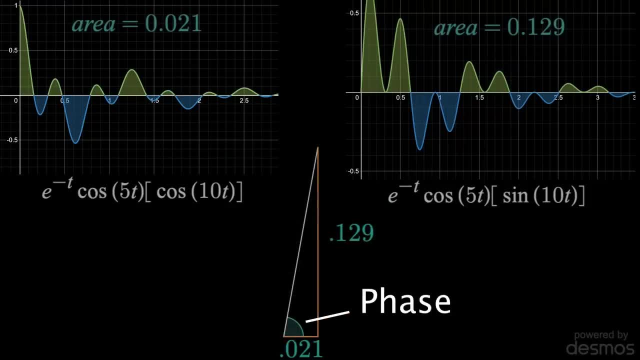 to those areas that we see here. if that phase is close to 90, like it is right now, then the times cosine omega t plot on the left has much less area than the sine omega t1 on the right. visually just means that the bottom length is really small compared to the height. i'll show the actual 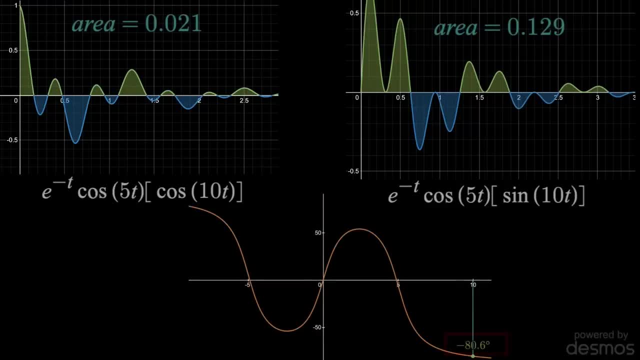 phase plot now, which has a value of roughly negative. 80 degrees at omega equals 10.. why is it negative, though? well, because that imaginary term from before, aka the height of the triangle, had a negative sign in front of it. essentially, we're in the fourth quadrant of the 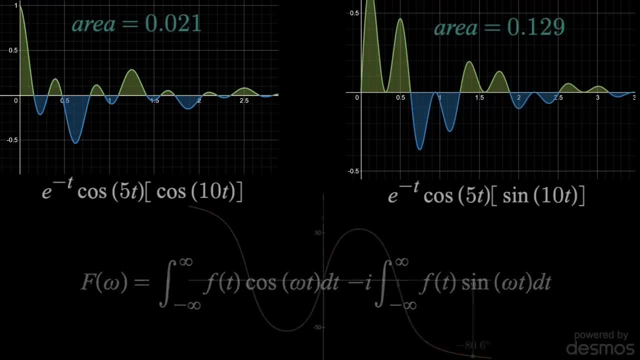 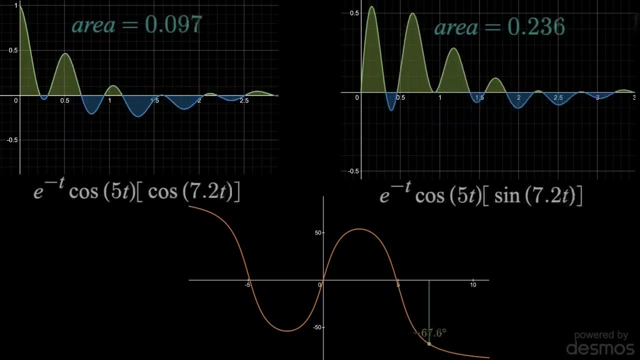 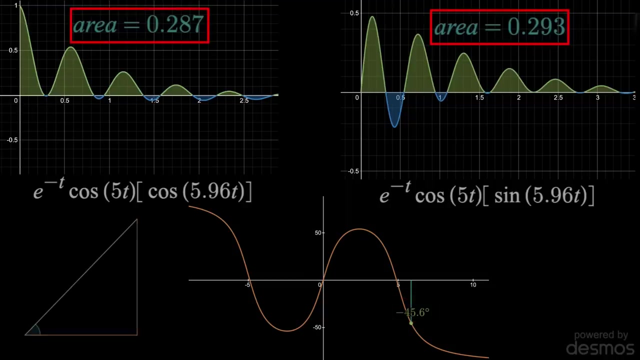 unit circle where negative 80 degrees is because of the negative y value. then as i change omega we can see some of the intuition behind the face, like when it's roughly 45 or negative 45 degrees, for example. then the absolute value of the two areas is roughly the same. as this corresponds to a 45- 45. 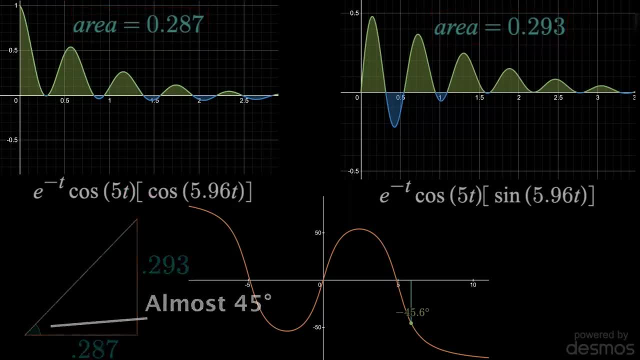 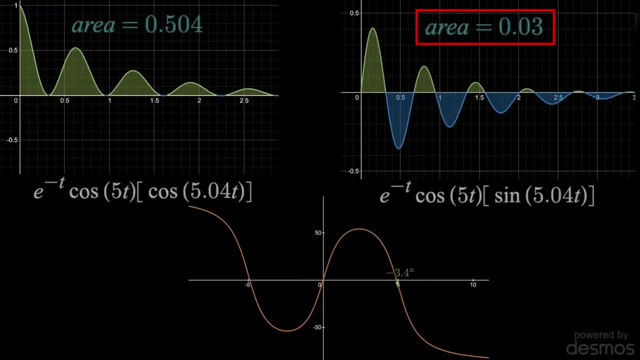 with two equal side lengths and if the angle goes to zero or close to it, then the sine omega t plot on the right will have zero or nearly zero area. essentially our triangle no longer has any height. then when we have positive phase values, at least between 0 and 180, 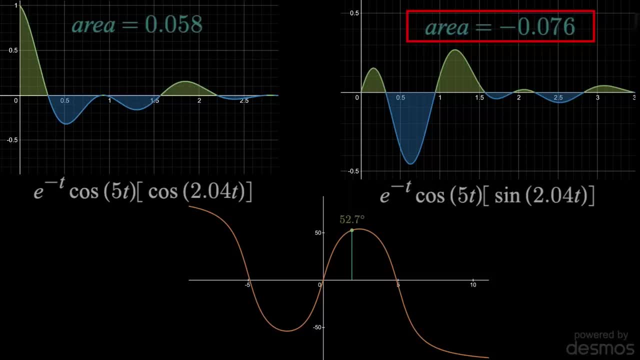 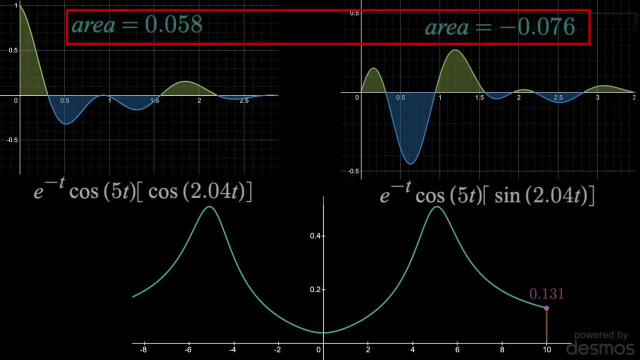 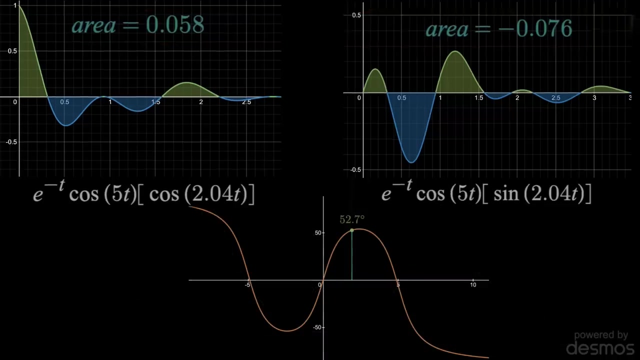 this corresponds to a negative area for the sine omega t plot. so in the end, the magnitude plot tells you how large the areas are when sort of combined, but you can just put through the Pythagorean Theorem. the phase plot, on the other hand, tells you relatively how big one area is compared to the other, as well as if either of them are negative. 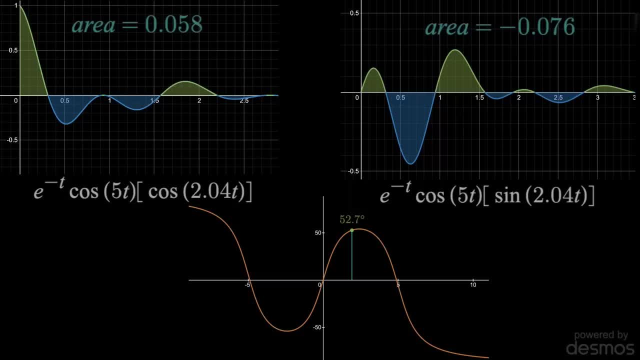 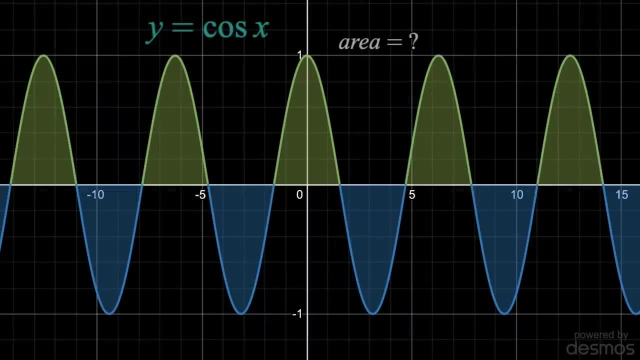 put these together and you get the full picture of the fourier transform. now let me ask this: what is the area under the entire curve of just cosine x, from negative infinity to infinity? well, i guess we can say it doesn't exist, because the area oscillates as the 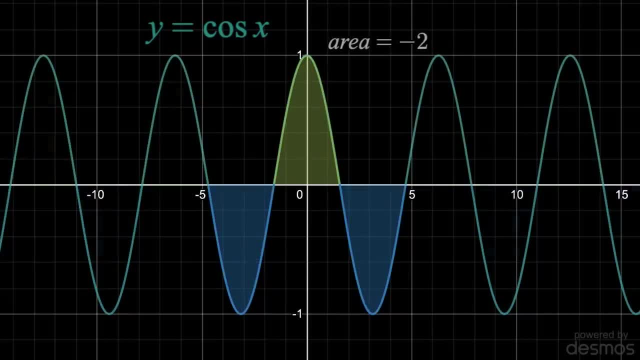 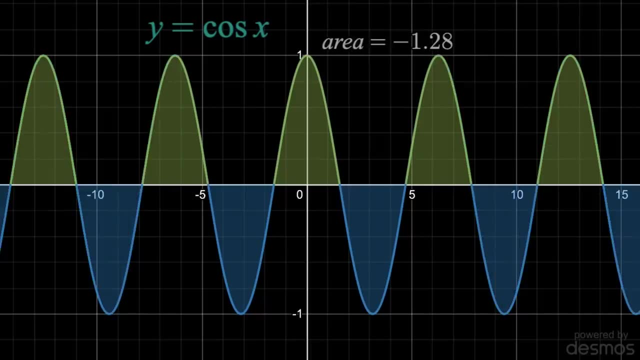 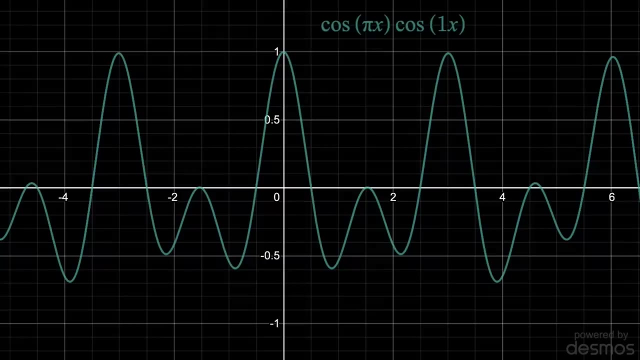 goes from zero to two, to negative two, and does this forever. it oscillates around zero, though, so it might not be right, but we're just going to call that infinite area zero. but now, what about two cosine functions multiplied together? i'm using two curves with very different periods. 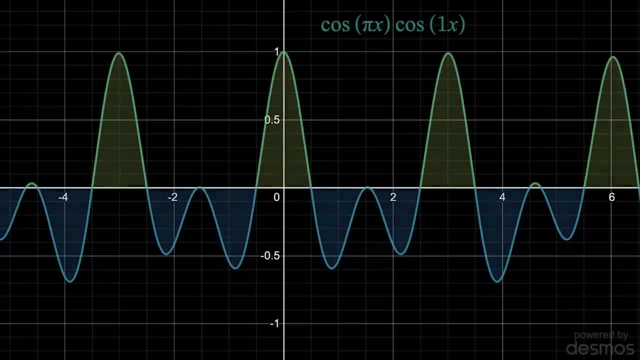 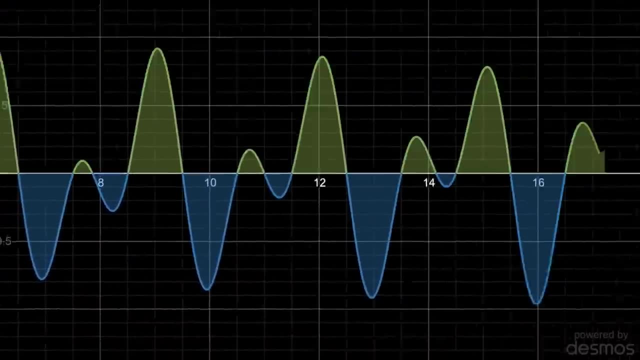 making for a strange looking plot, but even here the area is going to oscillate between two finite values. in fact, i'll move to the right and we'll see there are some regions with more green area and others with more blue, but just keeps going back and forth. so again, i'm going to call this. 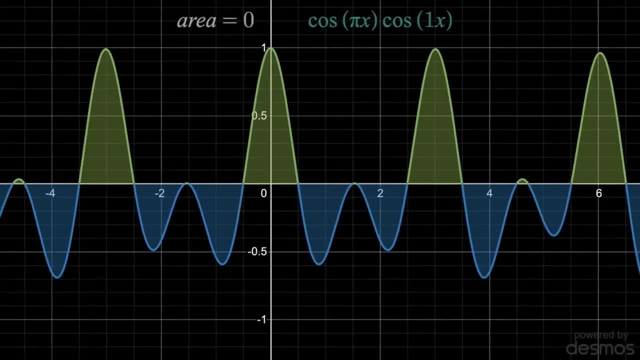 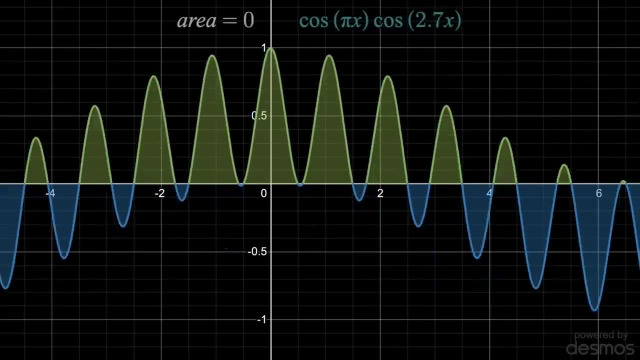 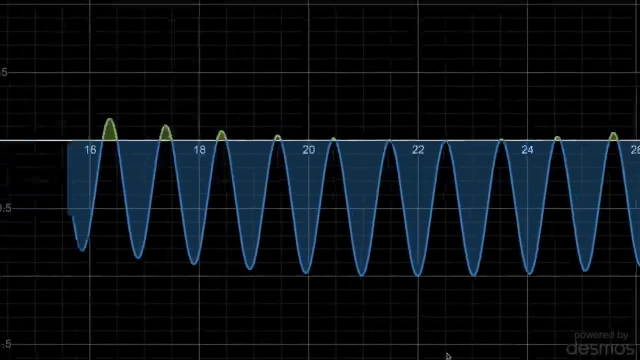 area zero as i change the period of one of those cosine curves, that area remains zero in that it oscillates and does not diverge. even right now, where it looks like the area may diverge as we move over, we still see that periodicity. however, once the two equations have the same period, and only at this time, 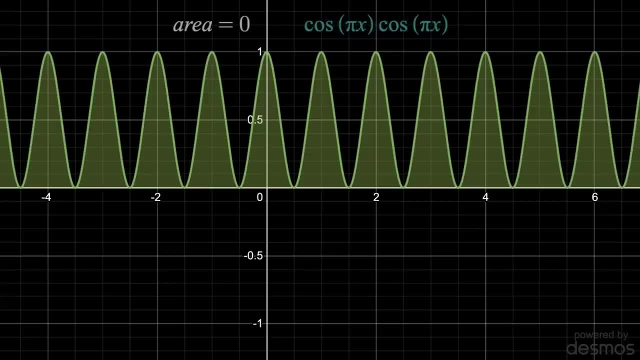 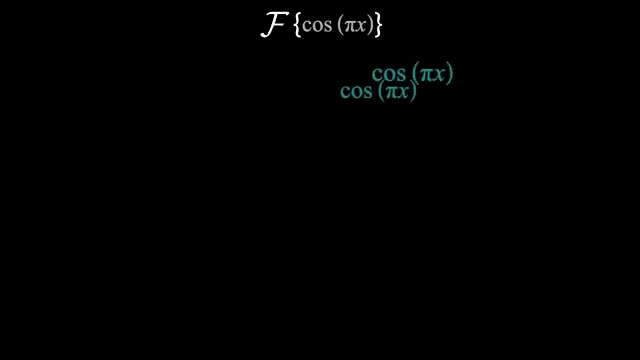 does the graph snap up a bit so we can see that the area is just above the x-axis, leaving us with an infinite area. this is just cosine of pi x all squared, which is why we only get positive values. now, if you were asked to find the 4a transform of, let's say, cosine of pi x from before, you know. 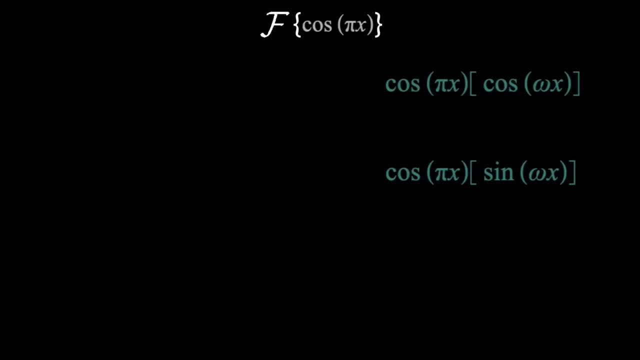 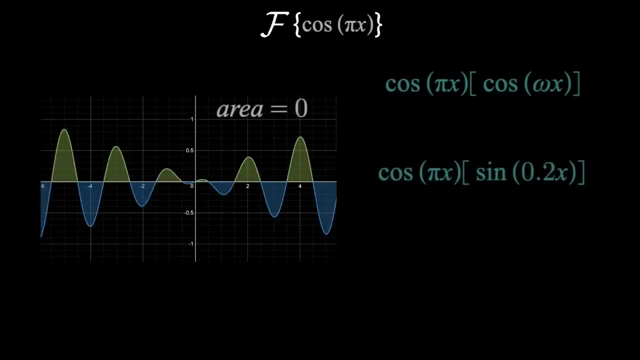 you're going to multiply that by cosine of omega x and sine of omega x and track the areas of each of those. the second one, though, will always have zero area. as i increase omega, you'll see that the green and blue areas are always equal and thus cancel. 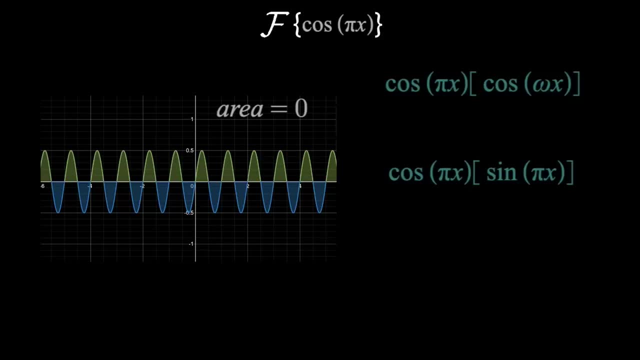 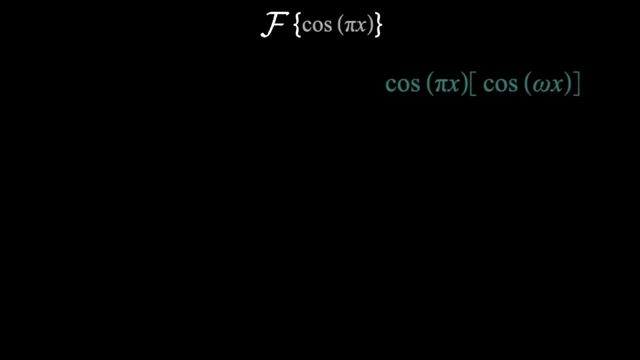 which happens because the curve is always symmetric about the origin, even when the coefficients are the same, we still see that symmetry and zero area. so i'm going to completely ignore this plot. for this other one, when omega equals zero, the associated graph has zero net area, which i'll plot to begin our fourier: transform magnitude. 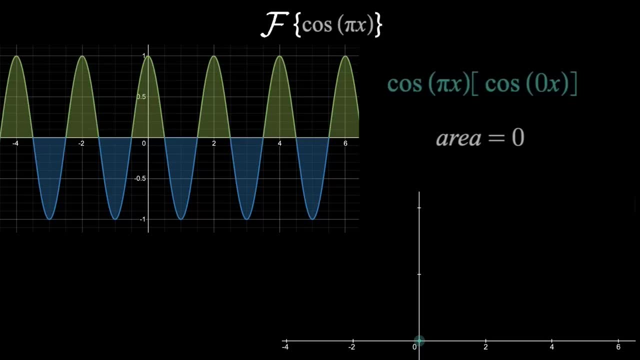 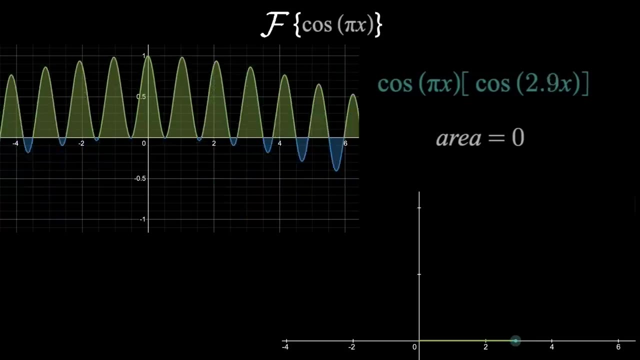 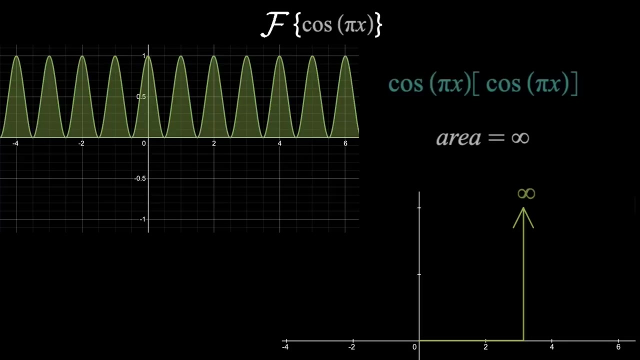 but even when we change omega, we'll see the same thing as before: a total area that just oscillates, which we say is zero. but at omega equals pi, the area all of a sudden jumps to infinity, which i'll represent on the magnitude plot with an arrow. and this only happens at omega equals pi, the angular frequency of our 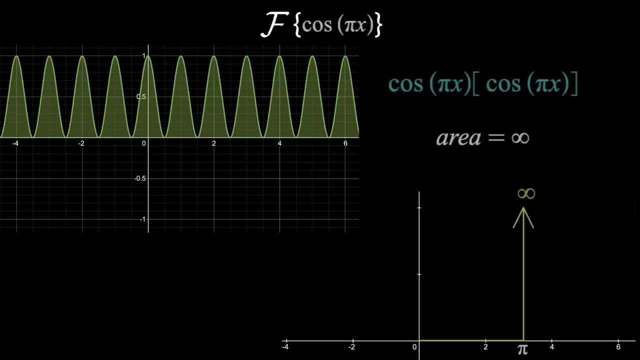 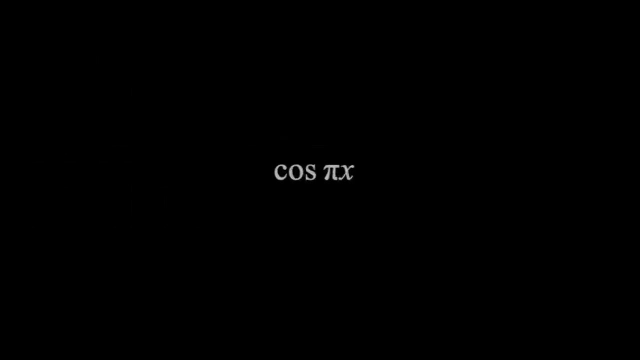 original signal. everywhere else the fourier transform, aka the area, is zero. so this would be the final fourier transform of cosine pi x, after accounting for that, even symmetry. this is the power of fourier analysis. it kind of scans your original signal for sinusoidal functions. 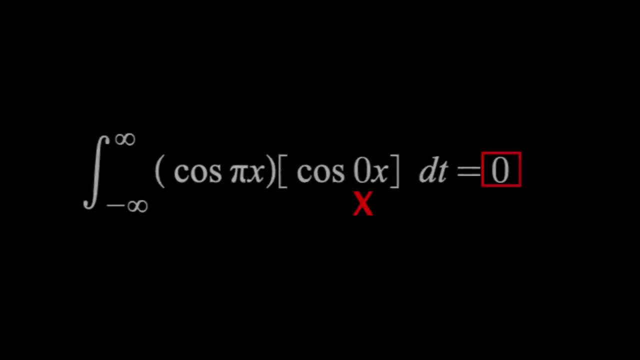 when it was on a wrong one, the output was zero. but once it found the right frequency it gave us a brief infinite output saying: hey, your original signal has a cosine of pi x within it. so really all we're doing is looking for the omegas that output an infinite area, because those tell us. 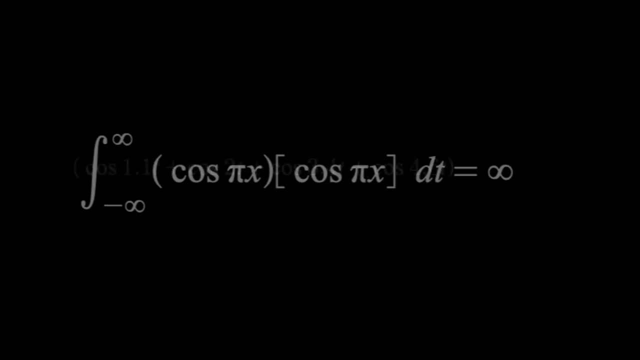 what sinusoids are in our signal. if we had a more complicated function and applied the fourier transform, well, we can think of this as four separate integrals, with each term multiplied by the cosine omega t. when there are no matches, then we get out zero area from everything. 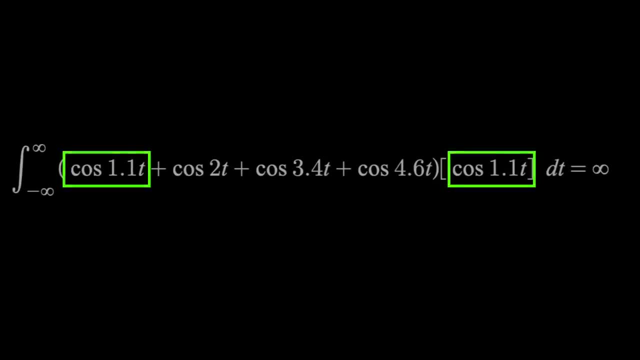 but once our scanner finds a match, we get that brief infinite area- and this will happen four different times, telling us we have four sinusoids in our function. now, of course, it's easy to see what sinusoids make this up. i mean they're right there. but if i gave you a square wave, for example, then it's. 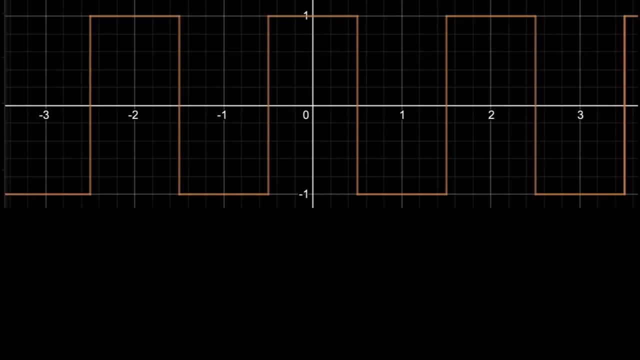 not remotely as obvious. however, with our scanner, we'll figure it out. i'll just call the square wave f of t and to find what sinusoids make it up, we just sweep the omega term and look for infinite areas. right now, i may equal zero. we're multiplying by one, which gives us an area of zero, equal parts. 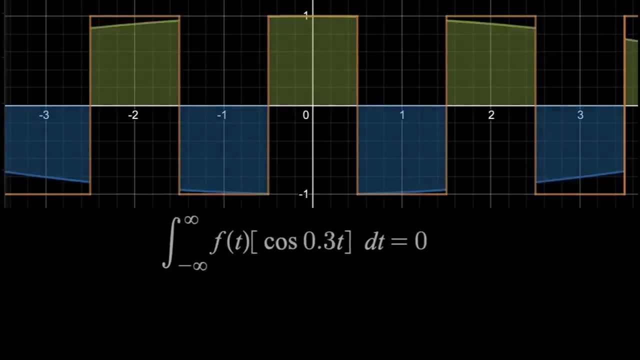 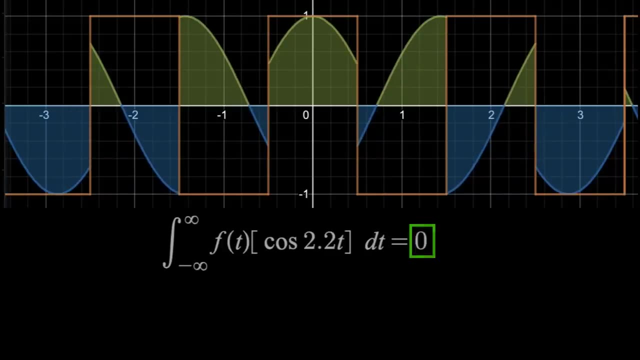 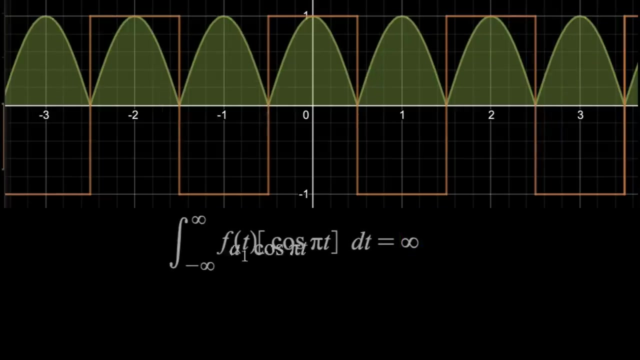 blue and green, so that isn't of interest. as i increase omega, this continues to be the case even here. if i were to scroll sideways, you see the blue and green regions all cancel. we get a sudden infinite area, which means we have found a sinusoid that makes up our square wave. 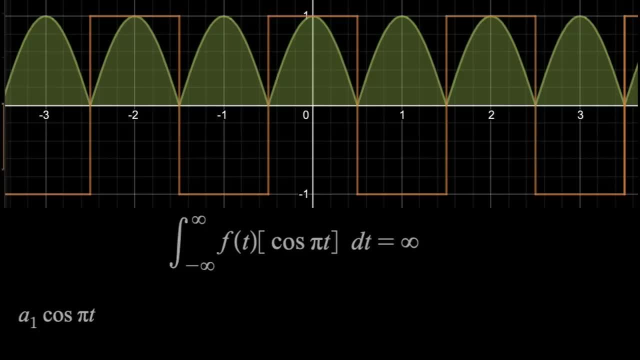 that was hidden from us at first glance, but the fourier transform found it. however, this isn't the only sinusoid in our function. we have to keep going. now i'm going to skip around. so if we jump to omega equals 2 pi, then the area will be zero. if you look closely, the blue and green regions. 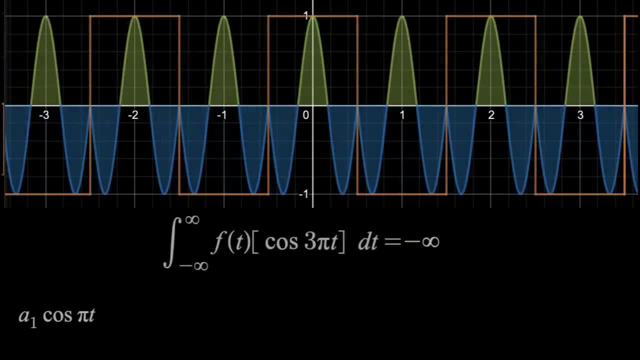 do cancel out. but when we go to 3 pi there's a continuous pattern of more blue than green. so we get negative infinite area, meaning there's a cosine 3 pi t also making up our function. but that coefficient will be negative for the negative area. as i keep going, it turns out only 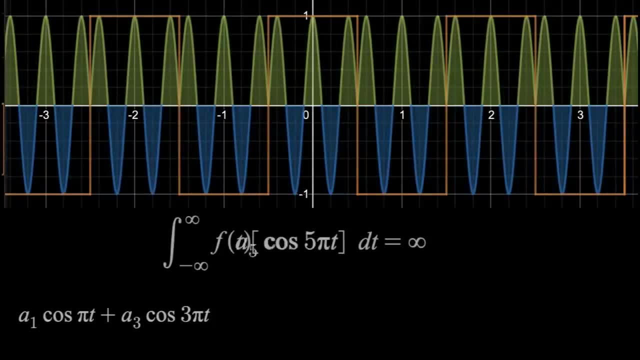 the odd integers times pi give us an infinite area, meaning that our square wave can be created by summing infinitely many cosine curves together with this pattern, which is the basic idea behind the fourier series. now, the last few minutes have been all about either having zero, 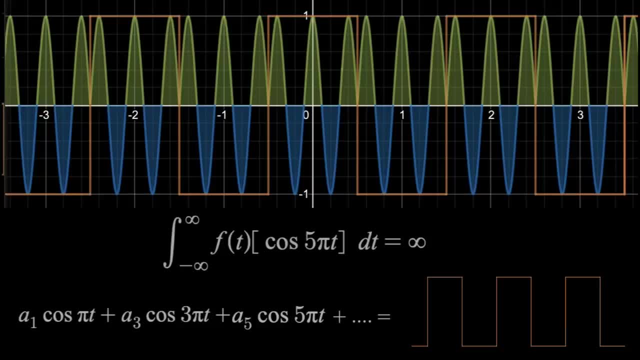 image and spoken graph, or the idea that we can't get the rest of the information from here because area or infinite area, which happens for periodic functions. but can we relate this to the earlier parts, when we were getting non-zero, finite areas like: is there anything deeper to the 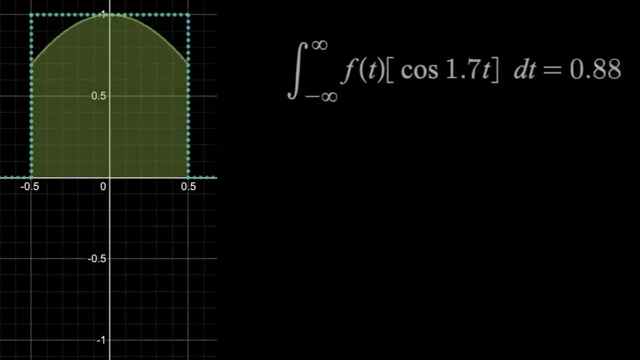 fact that we get this continuous change in area for the rectangular function from before. well, we could say that here, at omega equals 3, for example, our scanner found a cosine of 3t that makes up the rectangular function. the only problem is that we should be getting an infinite area. 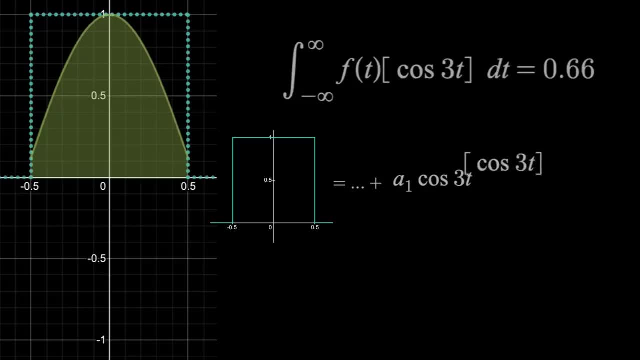 right now if that were the case, because when we multiply cosine 3t by itself we get that function with an infinite area. but if we let that amplitude get infinitely close to zero, then we could get a finite area, at least when we treat this kind of like a limit. so there is in fact a cosine 3t. 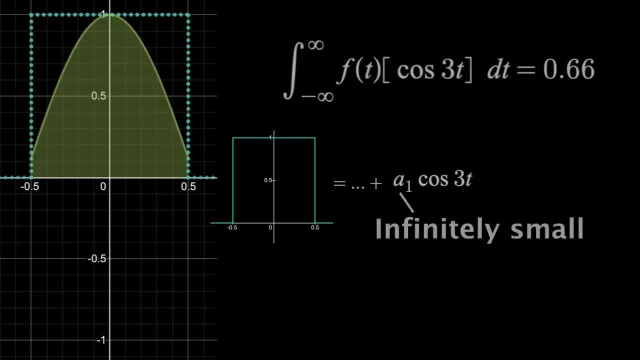 making up our rectangular function, but it's infinitely small. if we increase omega to 3.1, we still get a non-zero finite area, which means there's also a cosine of 3.1 t in our function with an infinitely small amplitude. this will be the case for pretty much every real 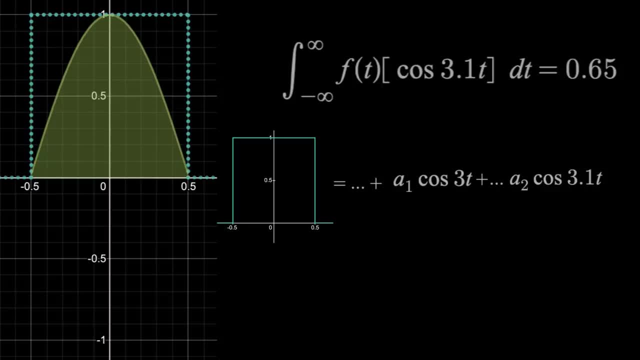 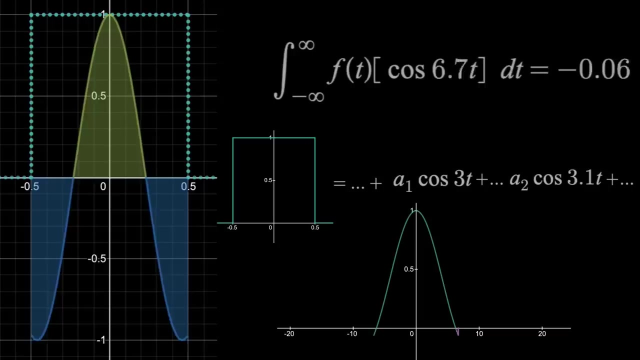 number, though, meaning we have to sum up an infinite number, a continuous spectrum of infinitely small sinusoids to make the rectangular function. and, when it comes to the visual intuition, instead of spikes we show an actual continuous spectrum of values representing all the sinusoids that make up our signal. 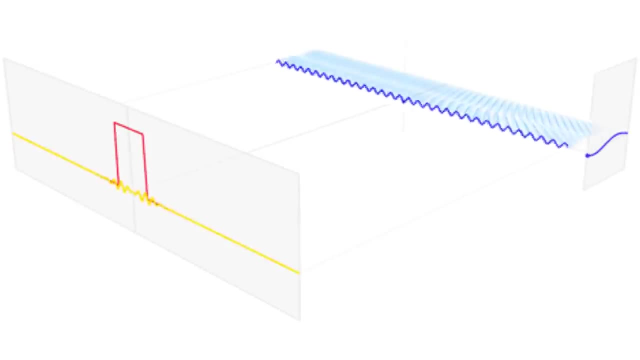 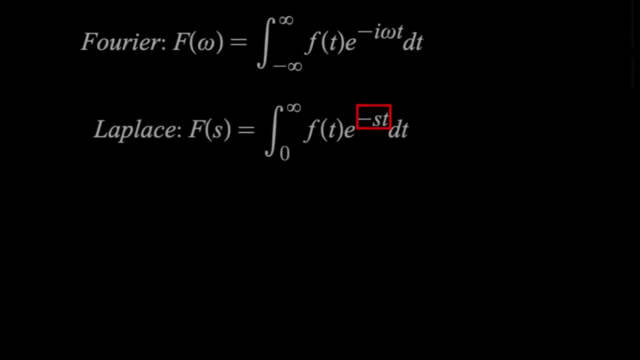 in this animation i've shown before highlights how that sum can create a real finite function. now i've done an entire video on the laplace transform, but real quick, since it's so similar. the biggest difference between fourier and laplace is the s in the exponent. 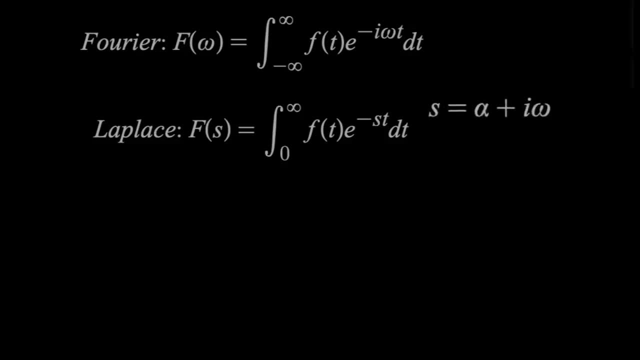 but that really represents alpha plus i, omega, which i'll put into the equation and then i'll split up the exponential as shown now. look, besides just having a zero as one of the limits, this is the exact same as the fourier transform, with one extra term. so, while fourier acted as a scanner, 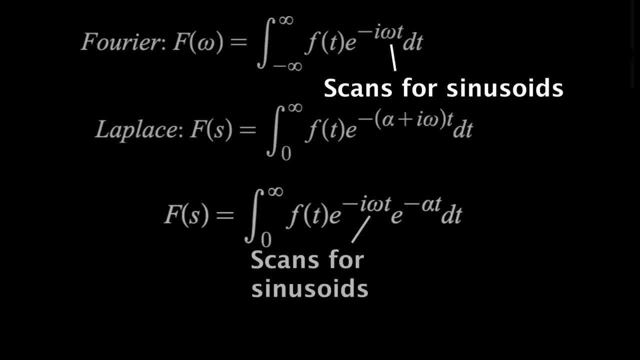 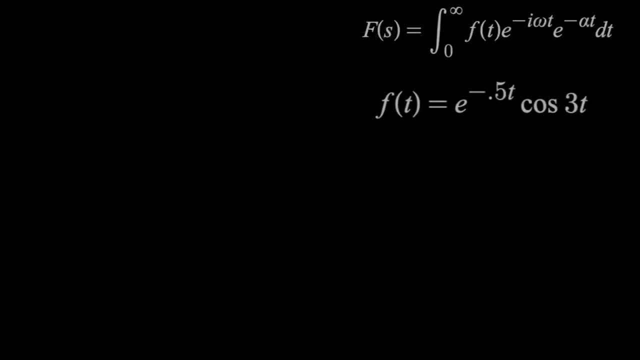 for sinusoids. laplace scans for sinusoids and exponentials in the same way, using areas. here let's say this is our function, starting at t equals zero. laplace says: multiplied by cosine and sine, omega t, just like before, but also including e to the minus alpha t, then find the area of both. 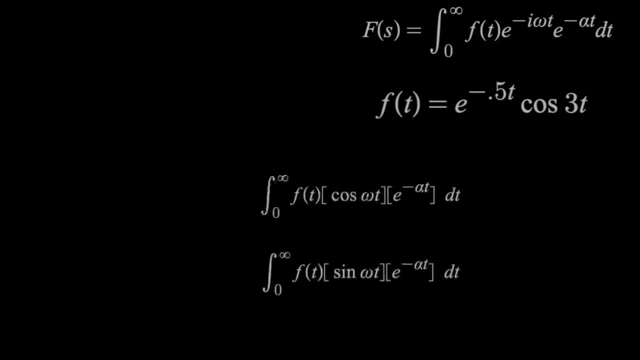 of those to make room, i'll put these over here next. aader's cube helps here, so apply primo until this form and the formulae areaka in case of over here. but I'm only going to plot the cosine omega t1.. Now we need two axes just for our Laplace. transform inputs. 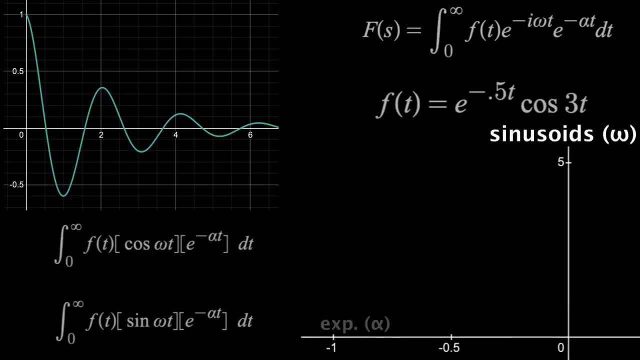 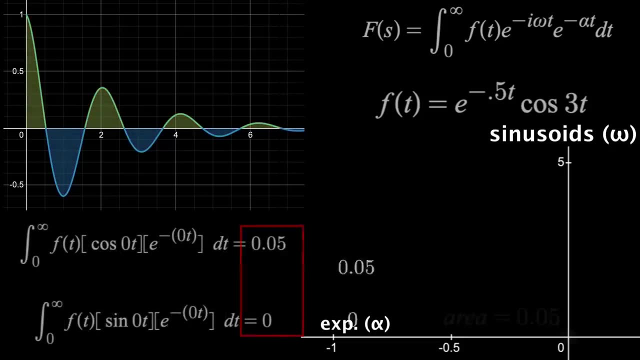 one for omega, aka the sinusoids, and another for alpha, or the exponentials, If we set both constants to zero. these are the areas, and I'll write that magnitude above the point zero, comma zero. Now, first I'm just gonna change omega. 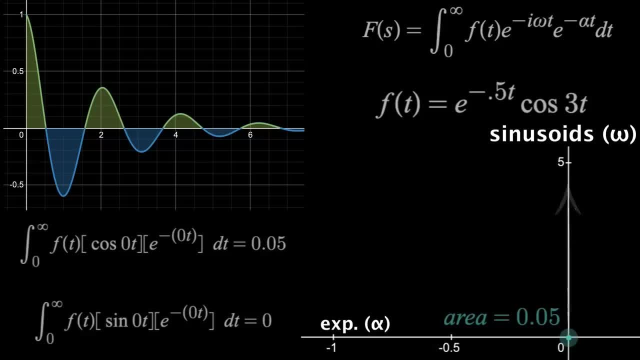 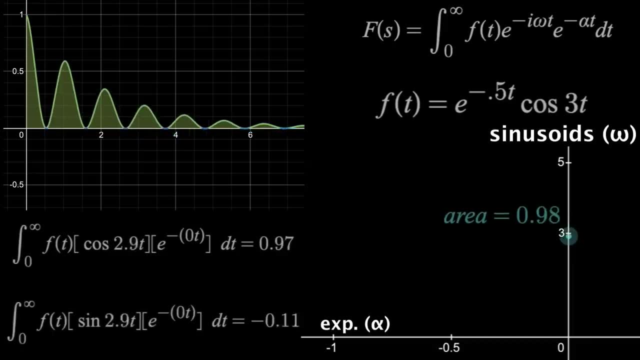 which will move the point up the imaginary axis and watch how the plot changes. Once we get to omega equals three, it again snaps above the x-axis. so the scanner kind of has found the cosine of three t in the original function, but not really. 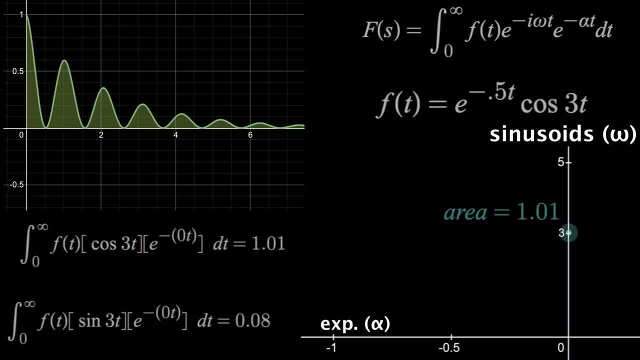 because we need an infinite area for that. There's no indication of anything special here from our output. But now I'm gonna change alpha or the exponential and I'll just remove the sine equation, since the area is negligible from here on. but again, watch how the plot changes. 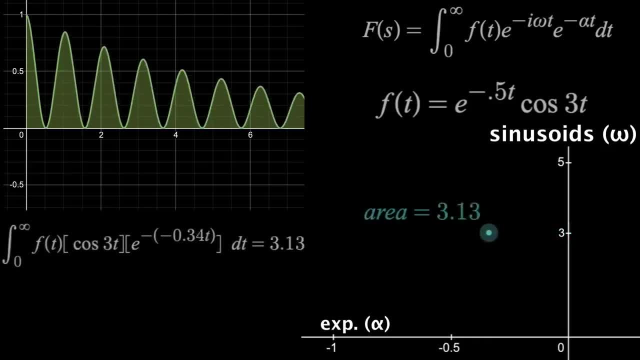 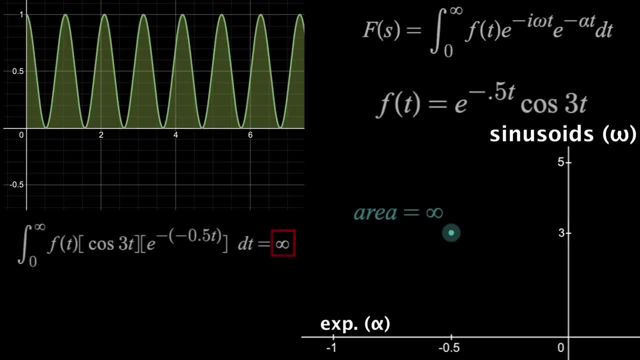 Once we get to alpha equals negative 0.5, there's no longer any decay and we do get an infinite area. That infinite area now means our scanners have found not only the sinusoid but the exponential in the original f of t. 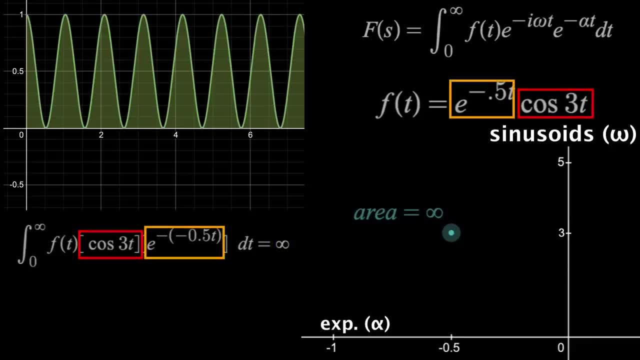 Just ignore the first negative in that exponential on the left. by the way, Graphically, these infinite areas are one of the only things we include on our plots and they're represented with an x. So for those who need to understand why this is so important, 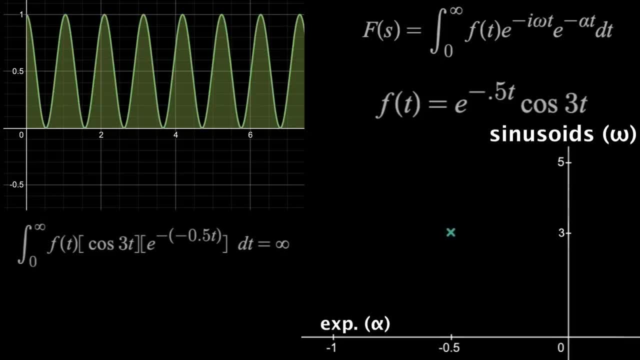 I'm gonna show you how to do it. First, we need to find the x-axis To understand pole zero plots. really, just find your poles and look at the associated y-coordinate and x-coordinate, because those tell you which sinusoids and exponentials. 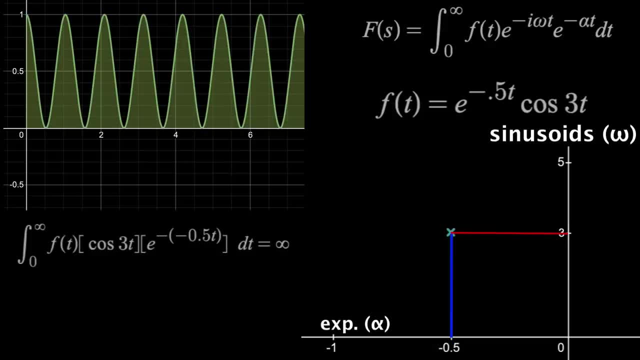 are in your equation, pretty much everything you need to know. We also plot values that give us zero area, but those aren't as important for our purposes here. The reason Laplace is so useful is because many systems like RLC circuits masses on a spring. 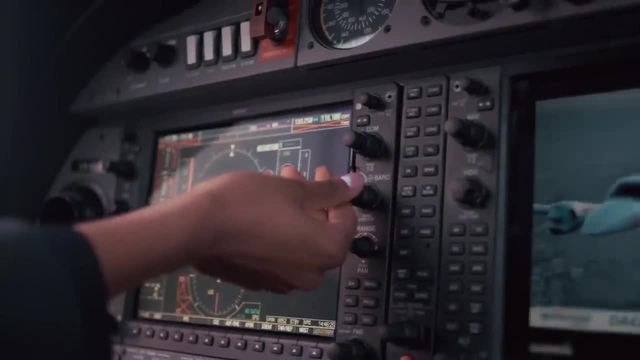 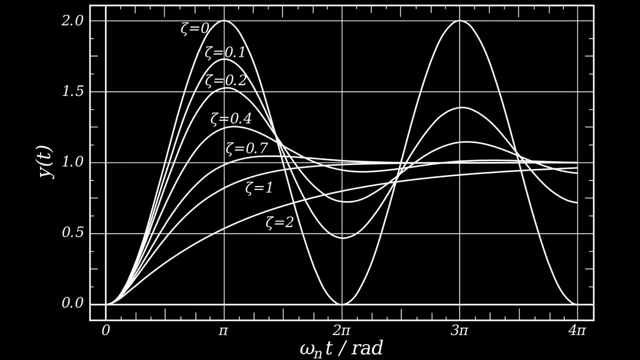 and just general control systems yield sinusoidal and exponential outputs, So we need something more powerful than the Fourier transform. in order to analyze these Again, I have an entire video on Laplace, including the 3D Intuition, which I'll link below. 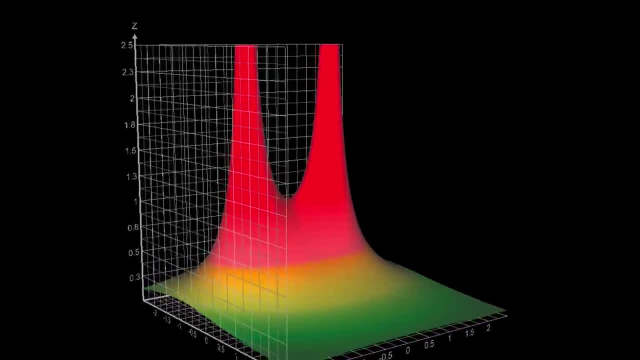 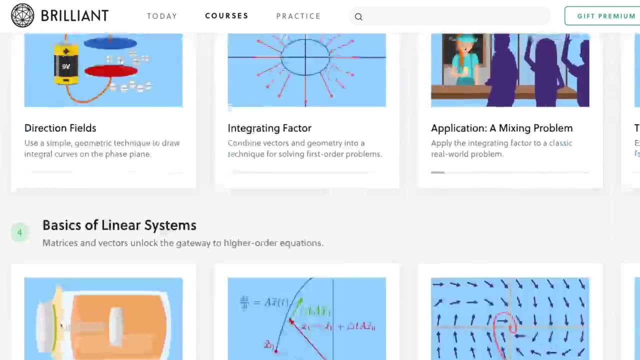 But if you wanna dive more into the applications of what we've seen here, I highly recommend checking out Brilliant's Differential Equations series. Their first course starts at the basics, but the second course is where you'll get into Fourier, Laplace and much more that you likely didn't learn. 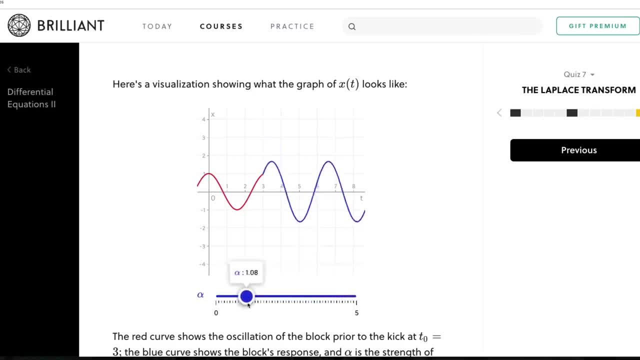 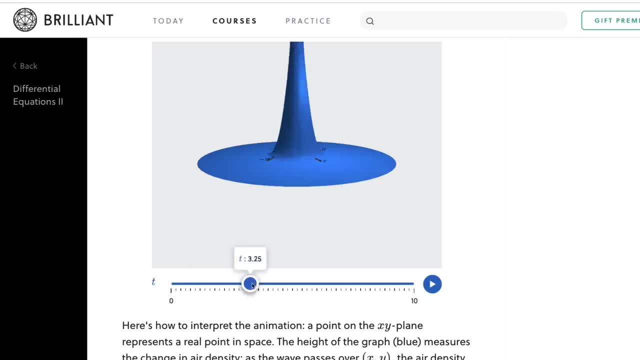 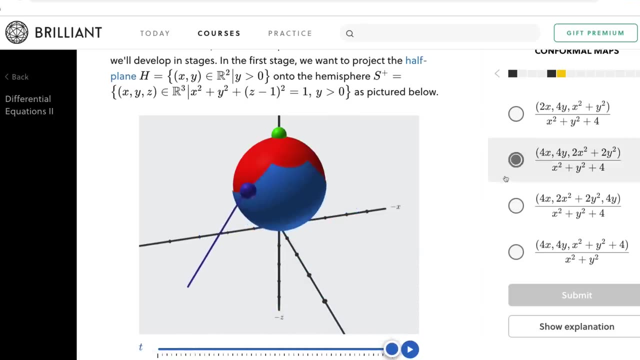 in an introductory differential equations course. Brilliant includes visual explanations, interactive exercises and constant practice problems to ensure you understand even the complex topics fundamentally and can successfully put them into practice. This is an educational platform that hosts a variety of courses from differential equations. 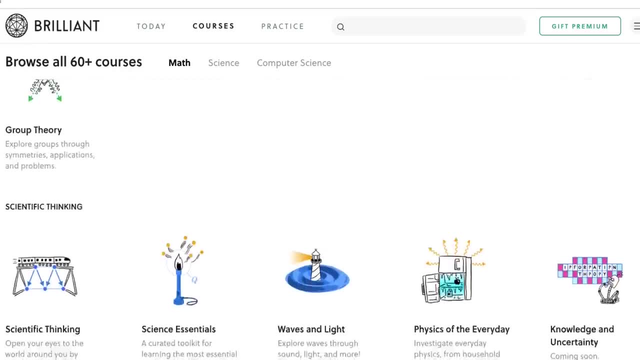 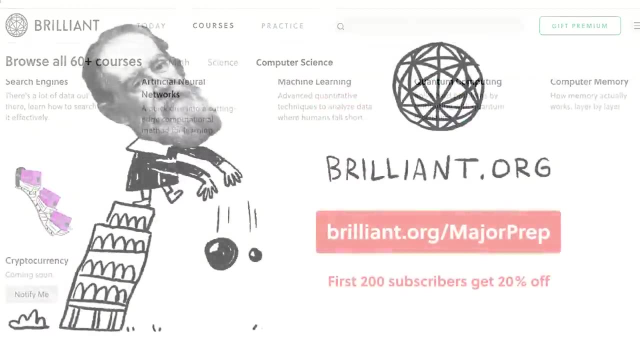 to vector calculus, to relativity and more for those looking to learn something new or just relearn old material. Plus, the first 200 people to sign up will get 20% off their annual premium subscription by going to brilliantorg slash major prep. 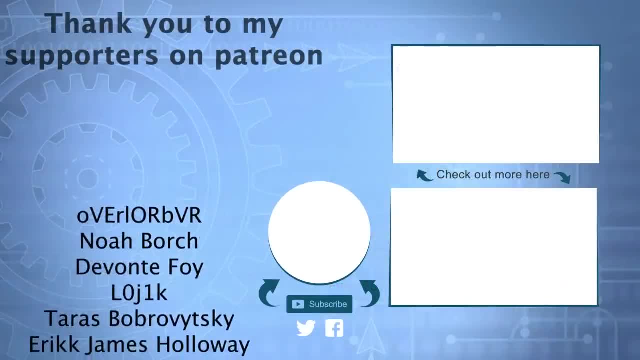 or clicking the link below, And with that I'm gonna end that video there. If you guys enjoyed, be sure to like and subscribe. social media links are down below, and I'll see you guys in the next video.